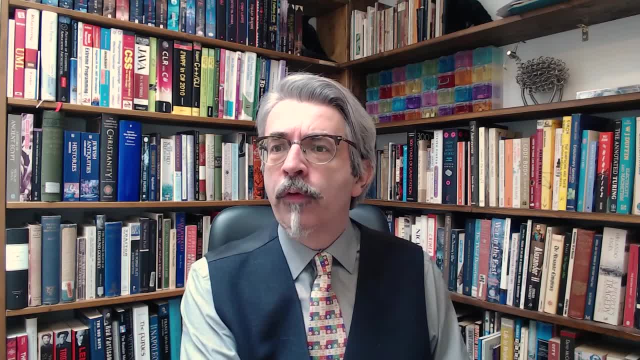 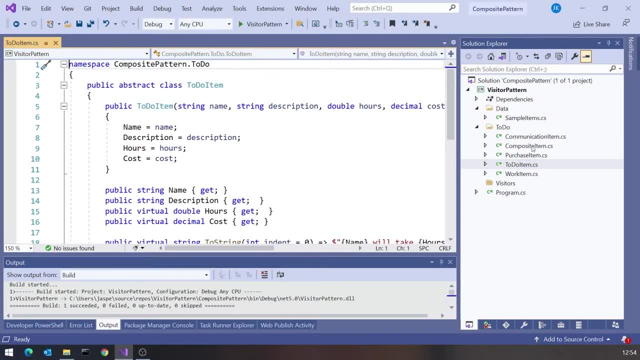 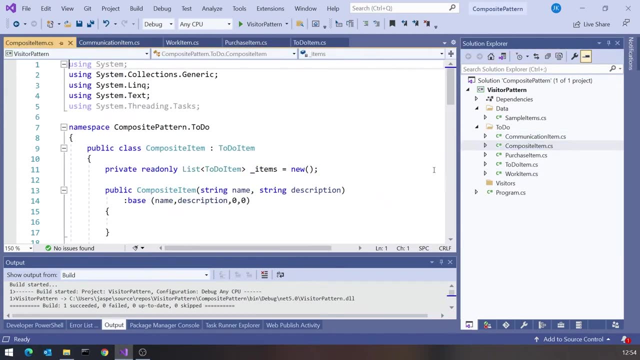 what we'll use it with for this demo And what we had from last week was a structure looking like this, where we had our Composite with the To-Do Item base class, We had Purchase Items, Work Items, Communication Items and then also the Composite that allowed us to put together in our program. 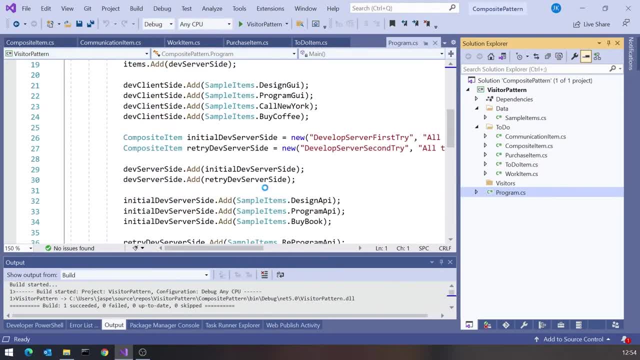 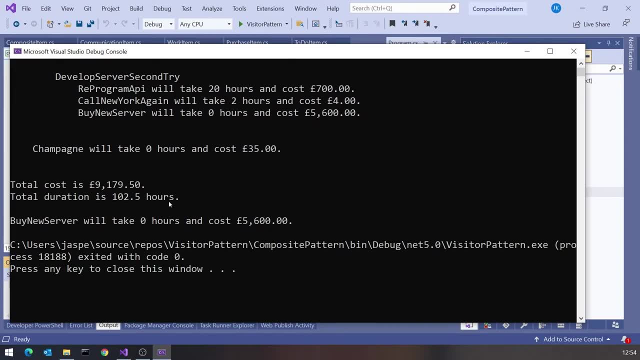 this hierarchical tree. And when we ran all that up we saw we could see the tree structure entirely displayed. We could see summaries of cost and duration. We could see we could find a particular item. So do have a look at last week's video if you're not familiar. 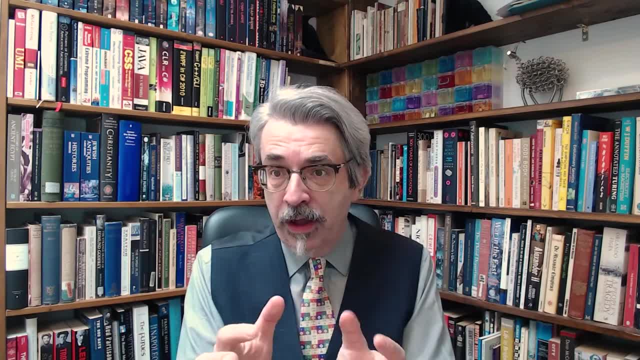 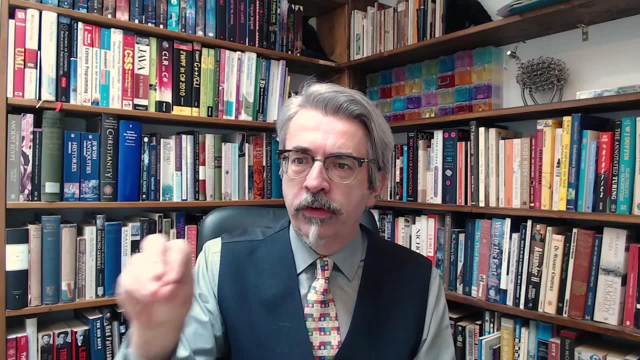 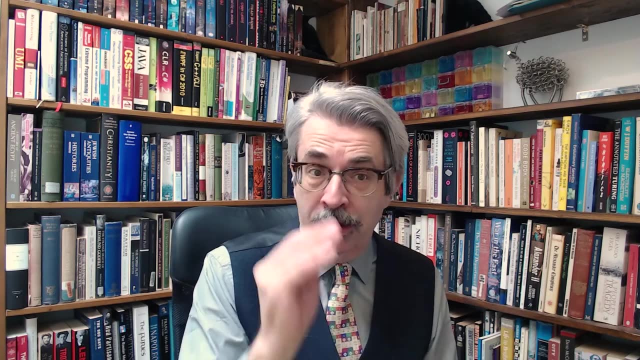 But the thing about the Composite pattern is it emphasizes the similarity between all of those different leaf nodes, In this case the Item nodes Work Item, Purchase Item and Communication Item, Because it operates really entirely through the base class and our base class just has the four. 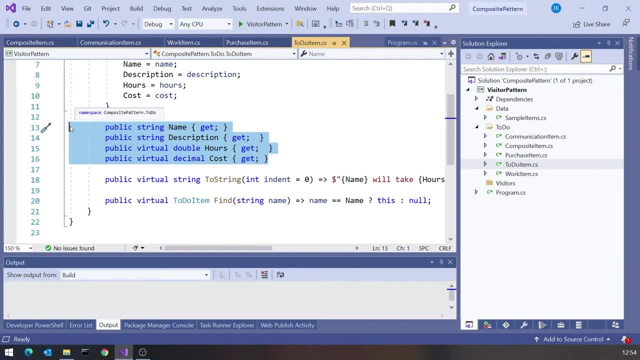 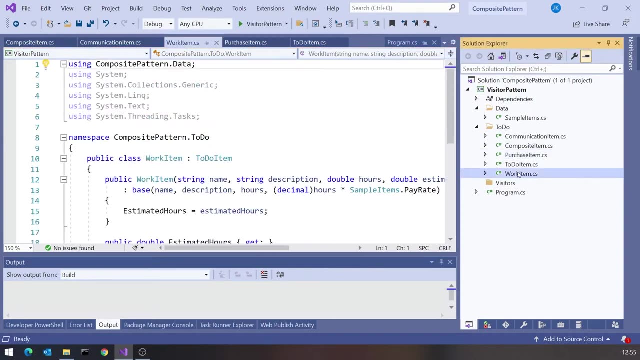 properties, Name, Description, Hours and Cost. But in reality you'll find that in these sorts of structures often in the individual leaf nodes you get additional features. So just by way of example, here we've added a Purchase Item as a Supplier and a Work Item as well as having the 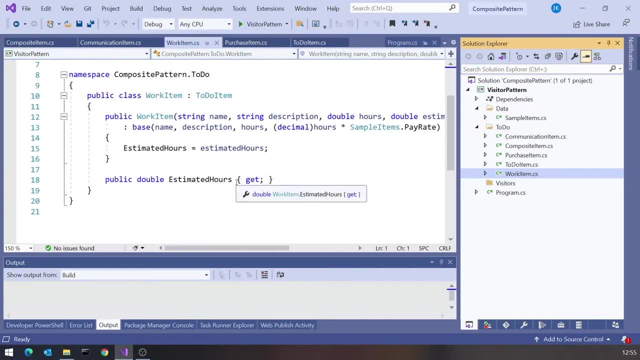 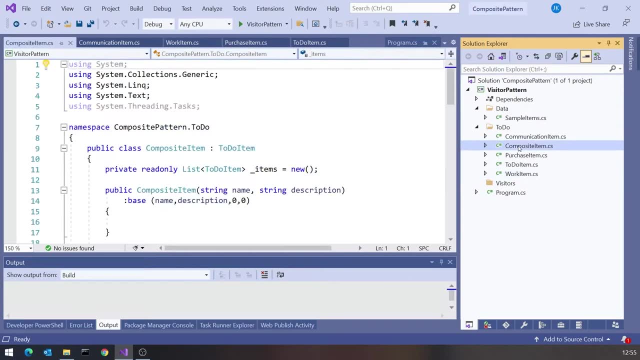 number of hours you actually worked, has the estimated number of hours that you thought you were going to work in advance. And as soon as we do that, we've got a problem because inside the Composite, the Composite only knows that it is dealing with To-Do Items It doesn't know about. 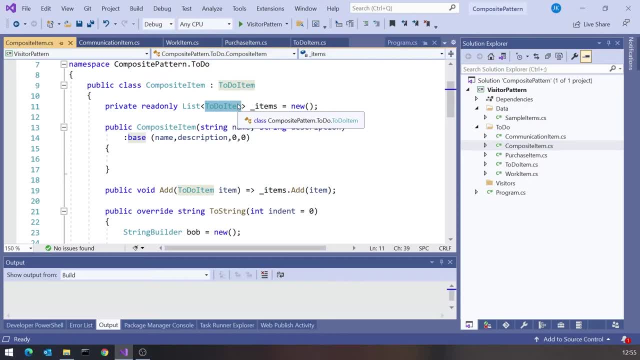 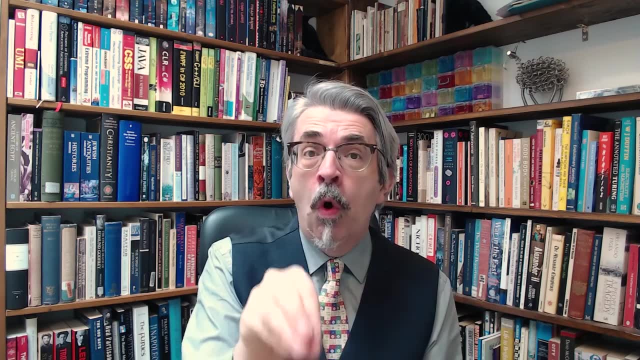 the derived classes. for perfectly good reasons: because we don't want to have to change it when we add a new derived class. But in fact, what that means is that the Composite itself is breaching one of our solid code principles- the first one, the Single Responsibility Principle- because it's doing two things. 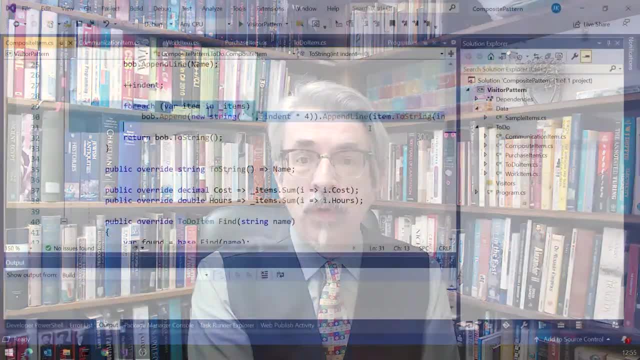 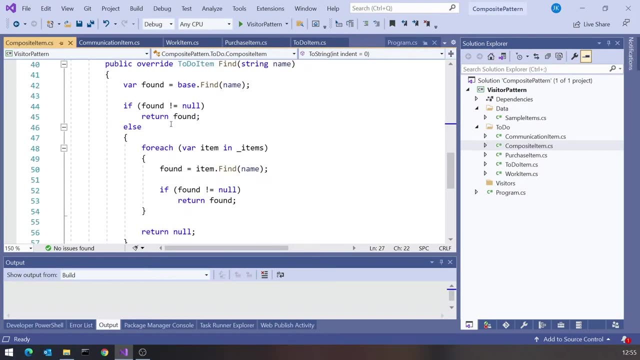 It's doing the iteration through the children, but then it's also performing the operations such as ToString and Find and whatever we may have. So in order to fix that, we need to split that out, to have a different class to do the job of actually calling the functions, And that's what 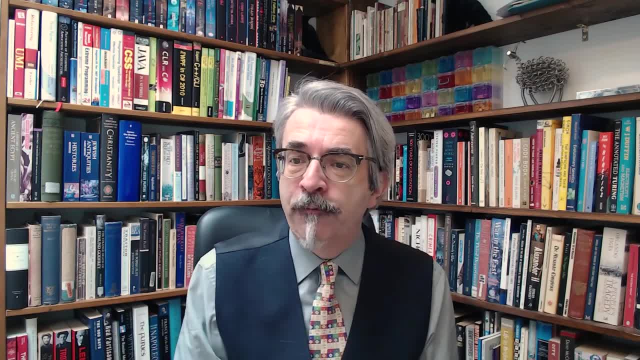 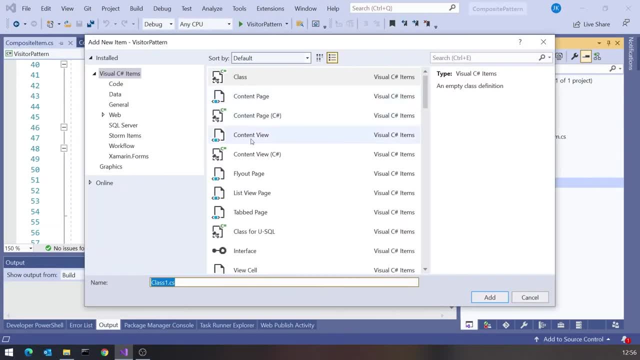 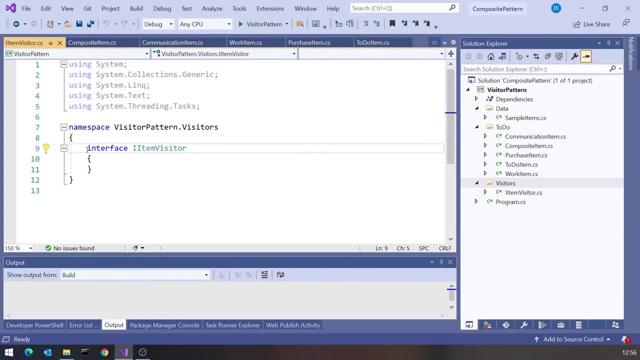 the VistaPack does. So I've put in here a folder called Visitors, and the first thing I'll do is add onto that a new interface that I'm going to call iItemVisitor, And then what I'm going to do with that is give that a method that turns void, is called Visit and then overloads each one of the concrete 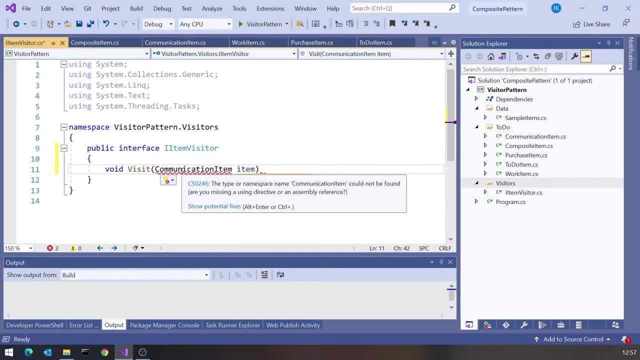 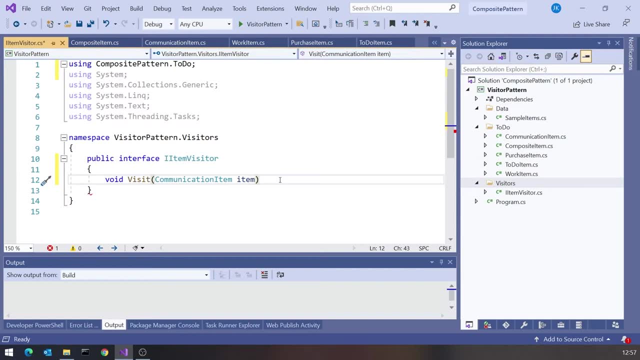 to-do item types. So we're going to have one of them for the communication item And also I'm going to use a nice little trick that we have in C-sharp 8 that we can have default implementations of interface methods, And I'm going to default all of these to do. 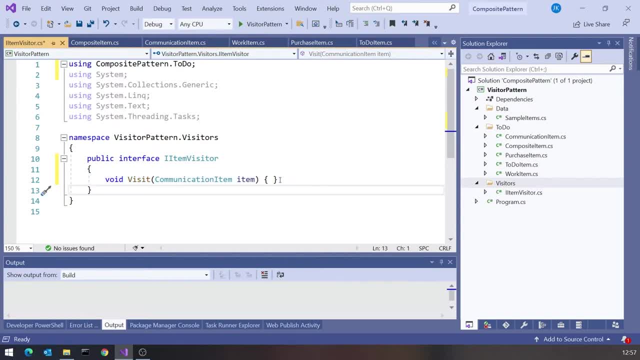 absolutely nothing. If you didn't have that feature- like we don't in other languages and didn't in earlier versions of C-sharp, if you didn't want to do anything, you'd have to override them in the derived class and make them do nothing there. So it's a bit easier, because quite a few 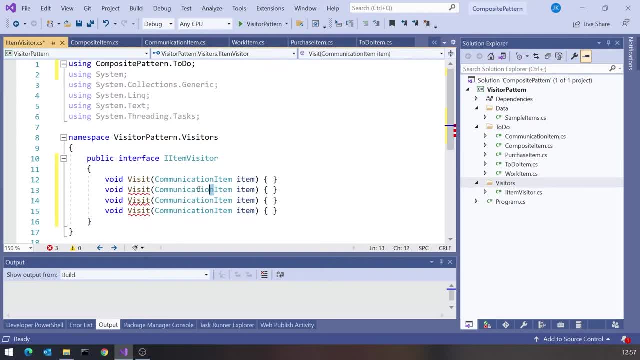 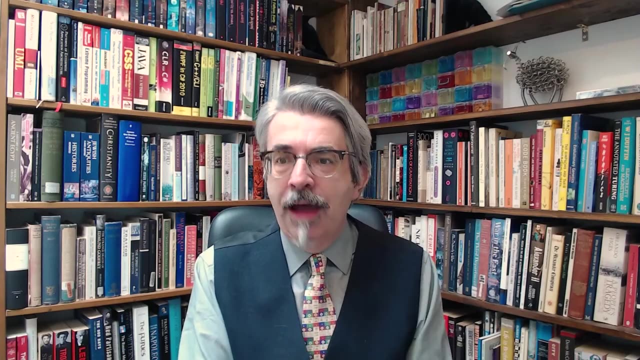 of these will default to doing nothing, to do it in the base class. So we have these for each of the different items: The work item, the purchase item, and also we have one for the composite item. So that's the interface that we have to have, And then also the change we have to make is on our 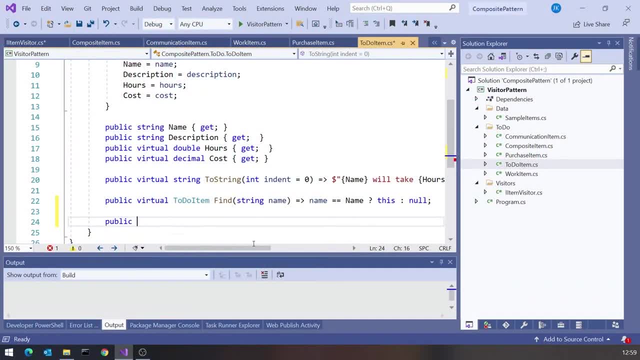 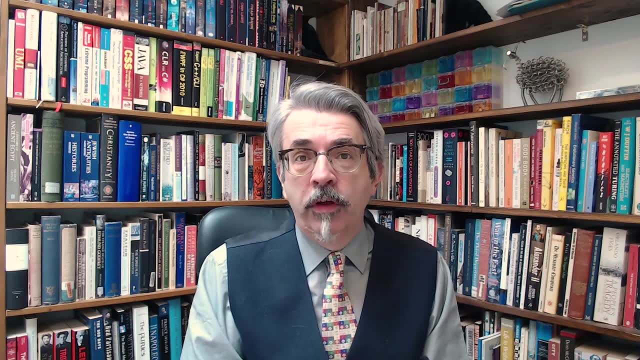 ToDoItem, And in here we're going to have a Public Abstract Void Accept method. The names of these methods- Visit and overload- are the same, So the names of the examples we're using are the two. You could really call them whatever you like, but the Gang of Four book and most 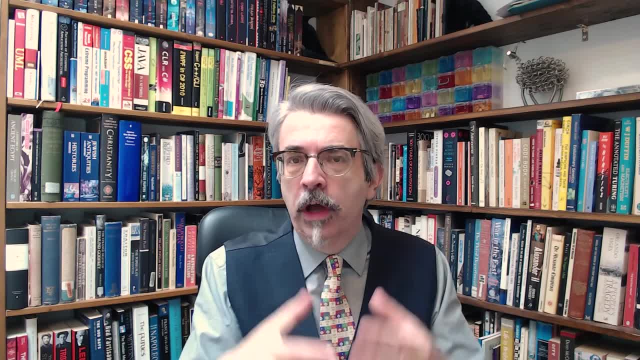 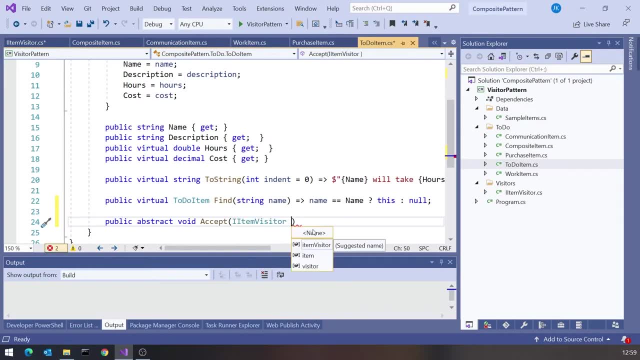 books, call them by those names, and so it just makes it easier for anyone looking your code to understand what's going on. But the Accept takes one of these item visitors and we'll just call that visitor and does absolutely nothing with it because it's abstract. And then what we have to do is, in each one of the 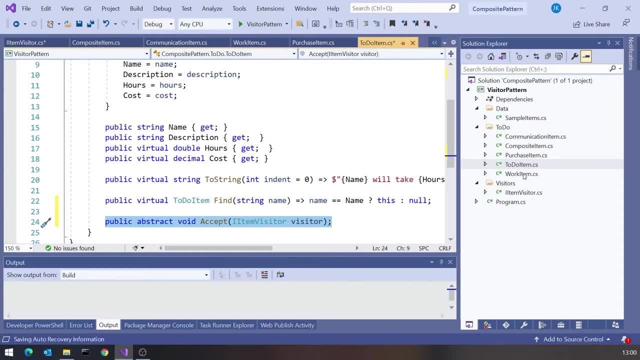 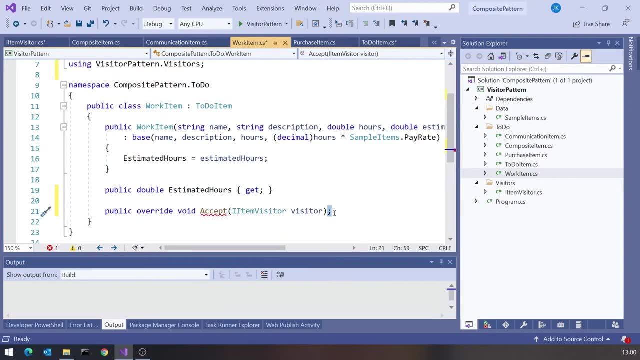 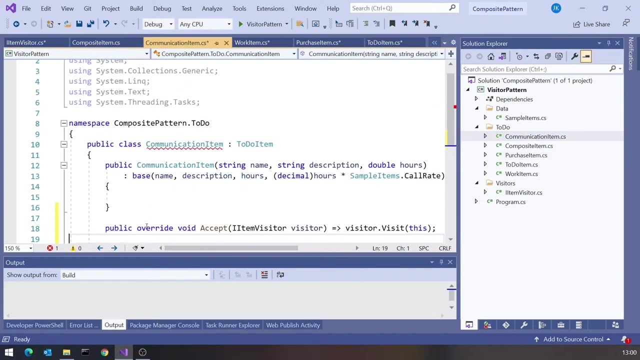 derived to-do items. we've obviously got to implement that And in the leaf nodes. that's pretty simple because all we need to do is implement that as visitorvisit and pass in ourself. So that code is exactly the same in the purchase item and the communication item Looks a bit repetitive that having. 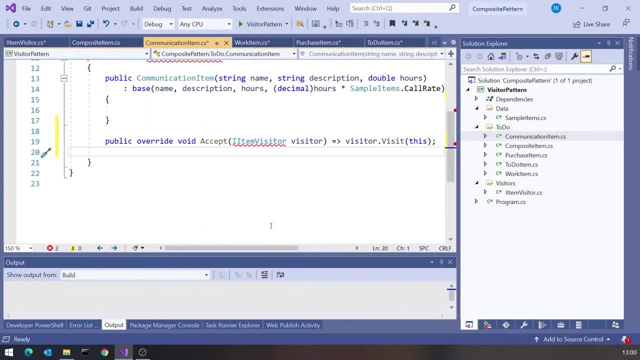 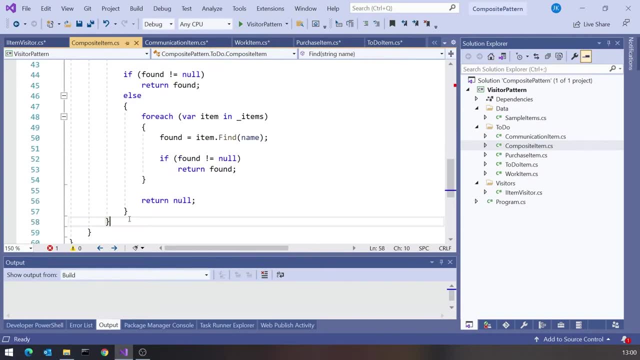 exactly the same code in all those places, but we'll come back to that in a little while. Then in the composite we've got to do a little bit more. So in the composite it still has to override that because it's derived from the work. 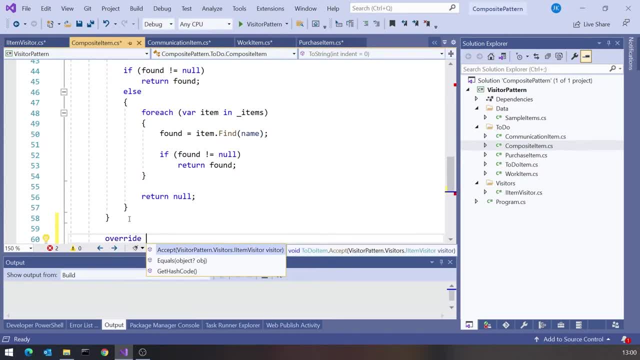 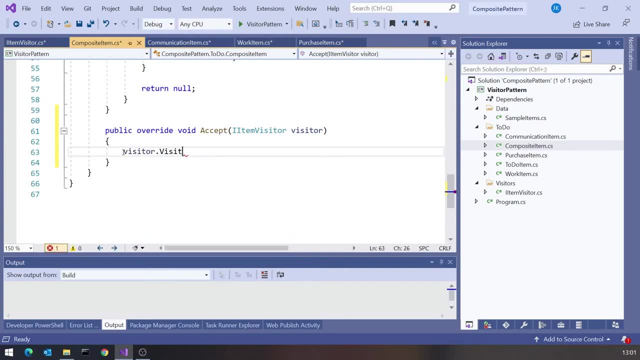 item. So here we say override of Accept, And then the first thing we do is exactly the same. We say visitorvisit ourself, But then, just like with every other job in the composite, we have to loop through. So we say for each var item. 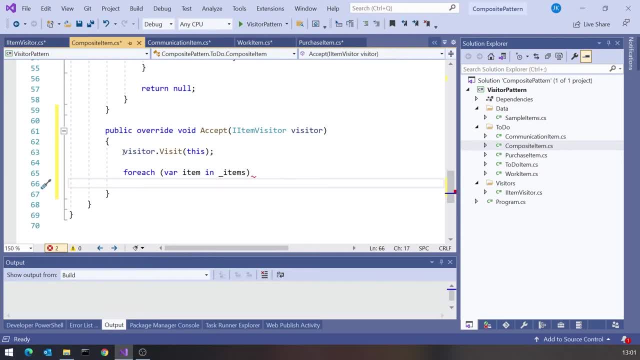 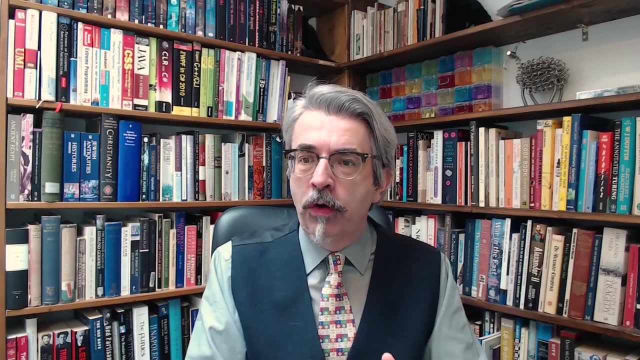 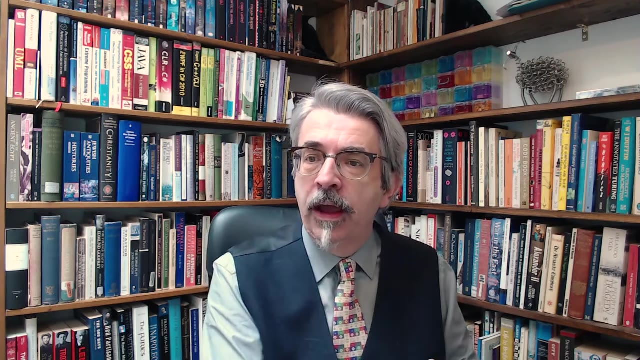 in items, Then on that we say itemaccept. But obviously, to make it do anything, we've now got to introduce concrete visitors to do particular jobs, And so, remember, these jobs are going to deal with the specific bits of data that we've put additionally on our concrete. 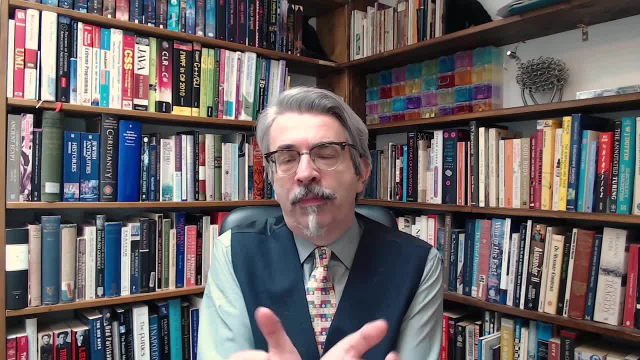 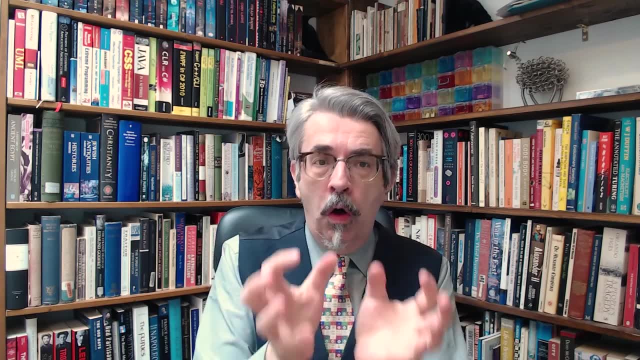 items. So let's consider estimated hours and let's suppose we want a visitor which is going to calculate the total overrun. So it's going to go through all of the items and if it's a work item it's going to subtract the actual hours from the estimated hours to give us the 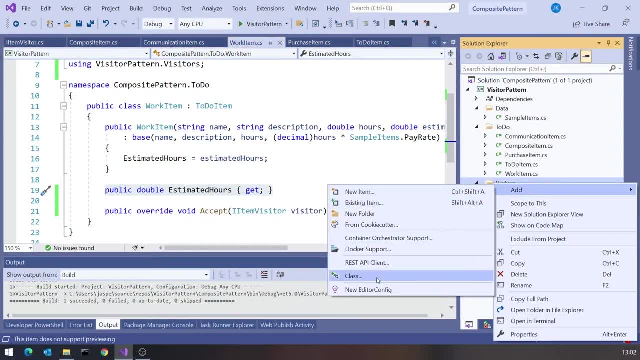 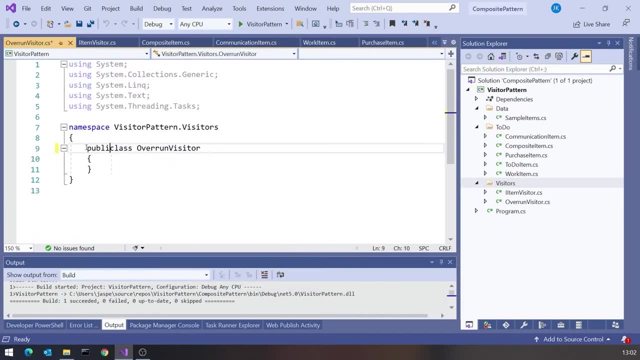 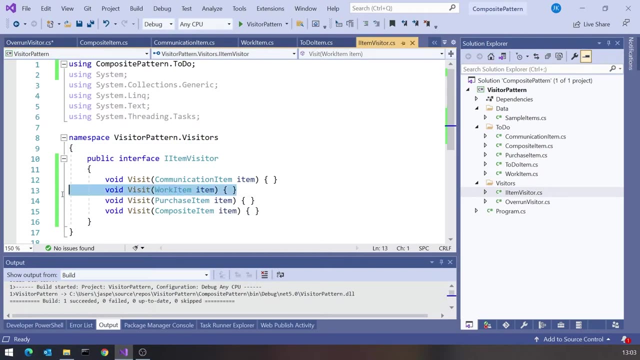 overrun. So that's what we'll do In the visitors. we will add a class and we will call this OverrunVisitor, We will implement the interface And then from the interface we're going to take that work item and that's the one that we're. 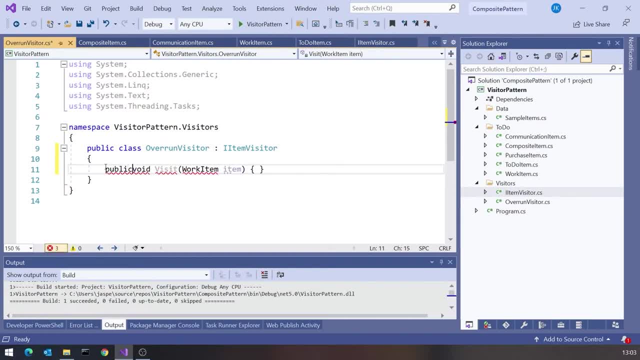 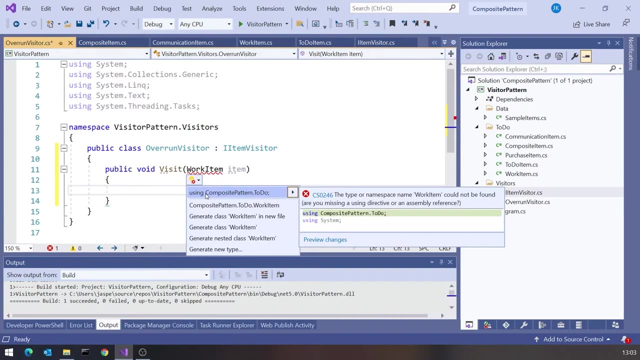 going to provide an implementation for. So that's the nice thing about having those defaulted in the interface. It means that for the other ones that overrun means nothing at all, for we can just ignore them completely, Whereas if we hadn't had that feature in the interface, we'd have had to just implement them directly to do. 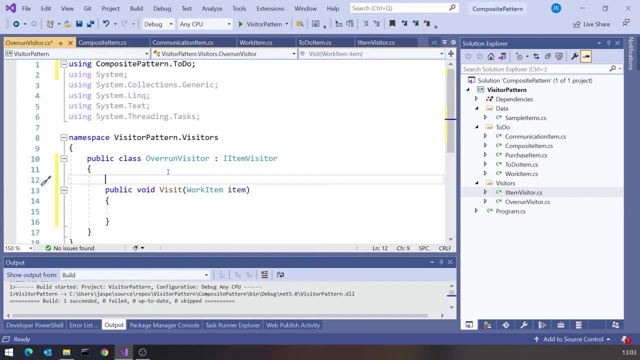 nothing. So we put that in there. and then also we're going to have a property of type double and we'll call this TotalOverrun And we'll give that a public get but we'll give it a private set, And then in here I'll simply say TotalOverrun plus equals, and then itemhours. 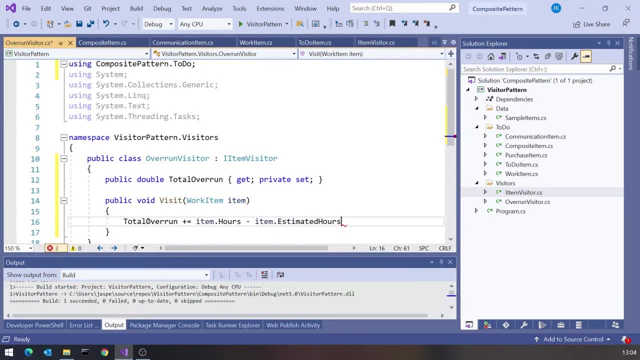 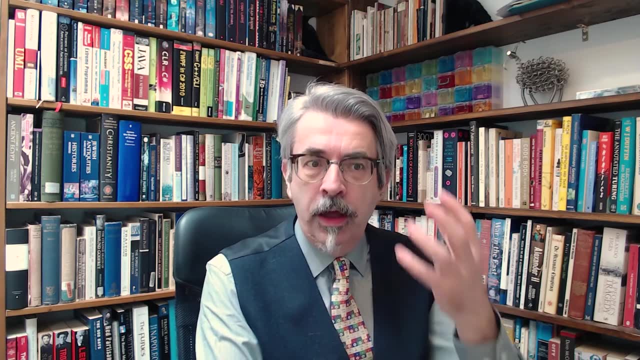 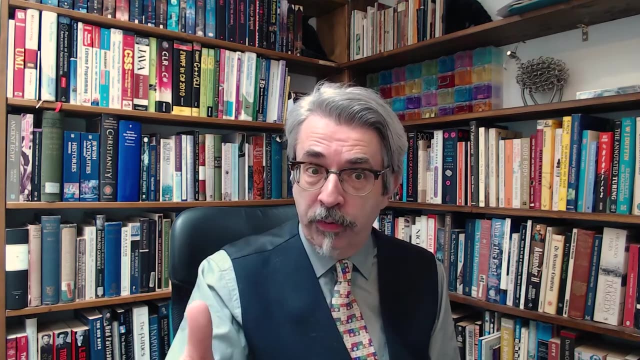 minus itemestimatedHours, And really that's it. That's the work done. So once the infrastructure is there, adding a new feature becomes just adding a new visitor, And that, of course, conforms with the open, close principle. Adding new functionality means adding new classes, not modifying existing classes, So that's that. 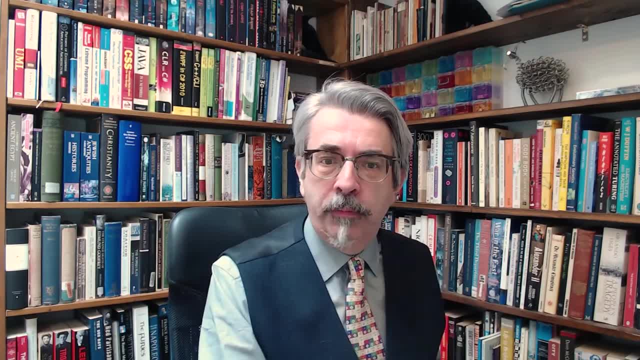 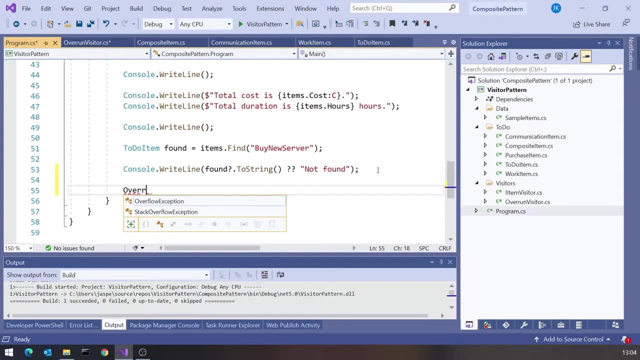 So we've actually fulfilled the first two of our solid principles now, And if we just use that, So what I'm going to do is I'm going to declare my overrun visitor, and then let's just call that ORV, And then I'll just take my route, which is: 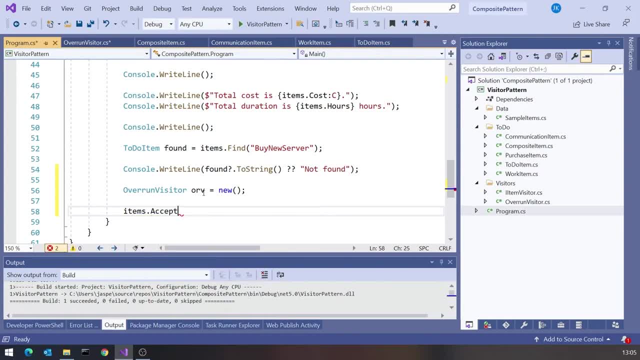 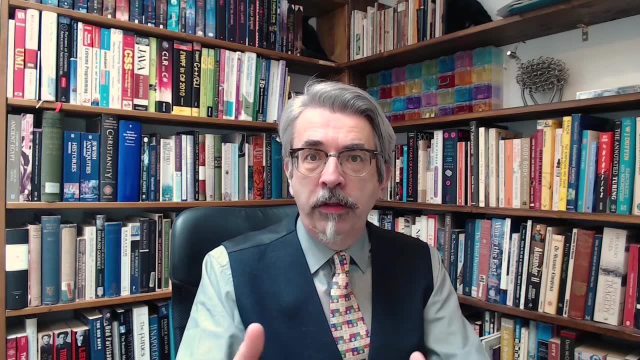 items which, remember, has the accept that takes a visitor. So we'll pass that in there. And then all that work of trickling it down through the composite structure, Finding the work items and adding up the calculation will be done for us. So all. 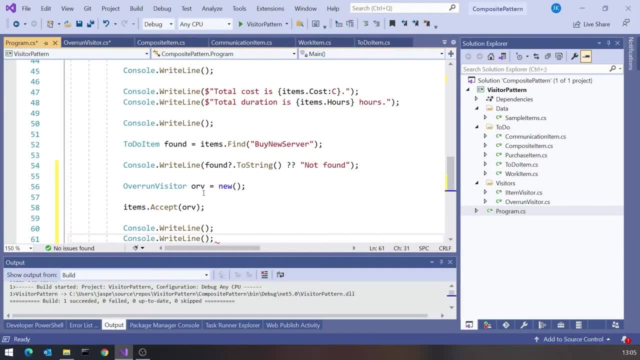 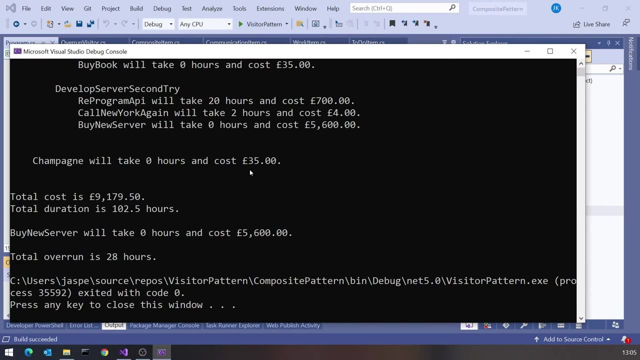 we now need to do is let's pop out a message saying TotalOverrunIs and then ORVTotalOverrunHours, And if we run that, then we can see we've got a total overrun of 28 hours. I'll leave you to. 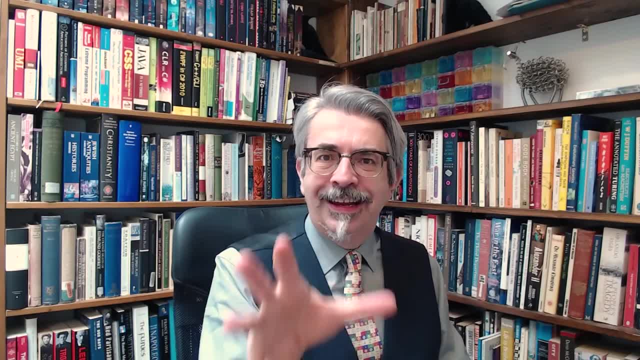 check that that's correct. But I think you'll agree it was fantastic as well. So that that's pretty much what we're going to want to see as we Jungel and, honestly, if we had things we could open up- outmatch, overrun- then hey that'd. 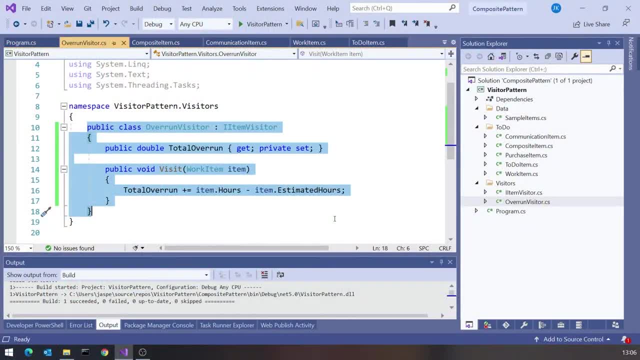 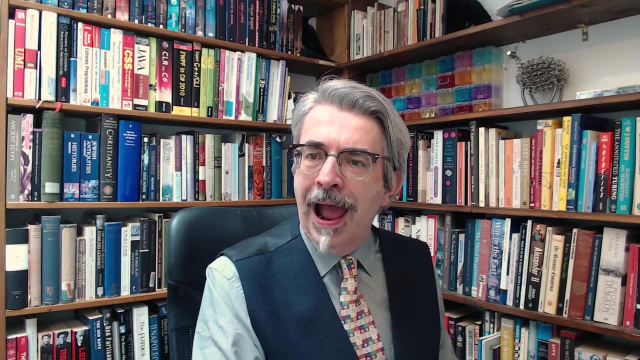 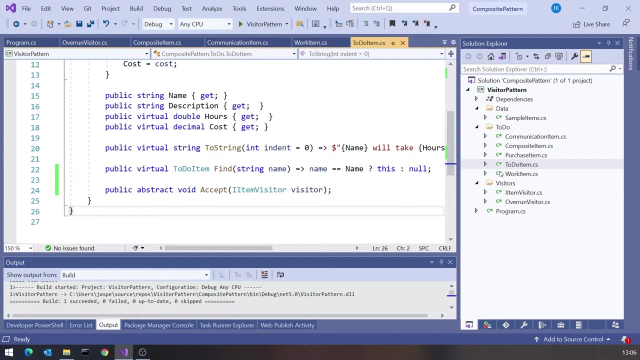 be incredibly easy once we had the structure in there, because that overrun visitor really just took no time at all to write. One slight improvement we can do here: Remember if we went back to our todo item, We declared that the accept was abstract and then we overrode it in each of the derived classes in exactly 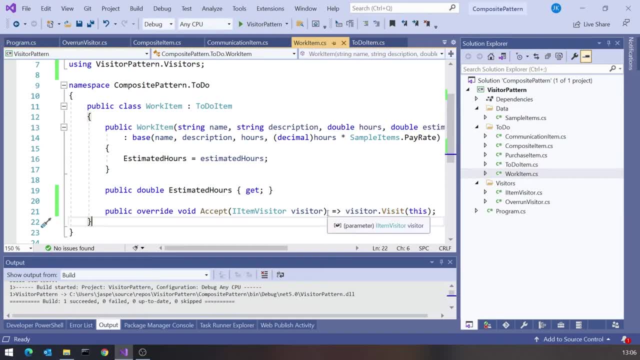 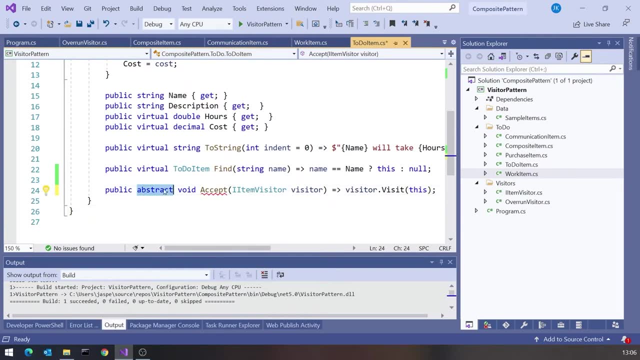 adopt VisitThis, And that was true for all of the leaf nodes. You might think: why can't we just have that implementation in the base class? If it's all the same, why duplicate ourselves? The reason being, though, that decision that's made with the VisitThis is done using overloading. 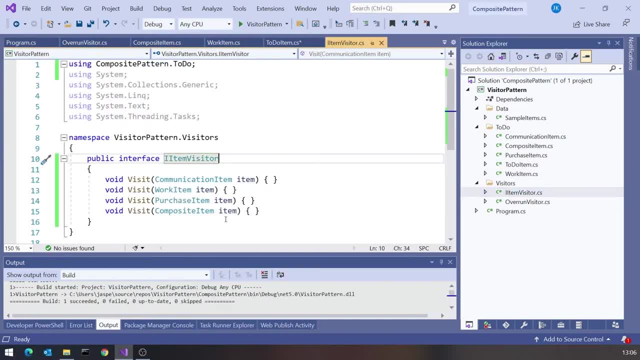 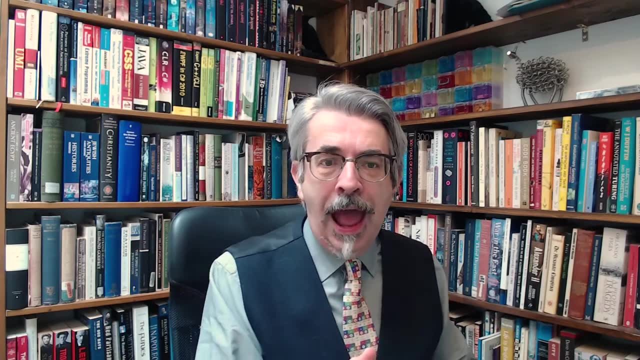 So, remember, our visit has four different overloads, and so that needs to work on an overloading basis, which is a decision that is made at compile time, not at runtime, And so in here, we don't know at compile time what actual type of to-do item this is. 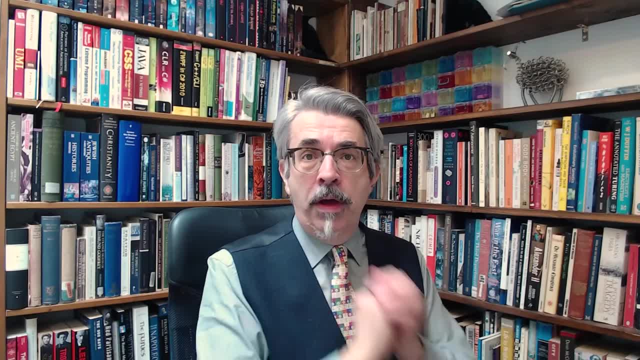 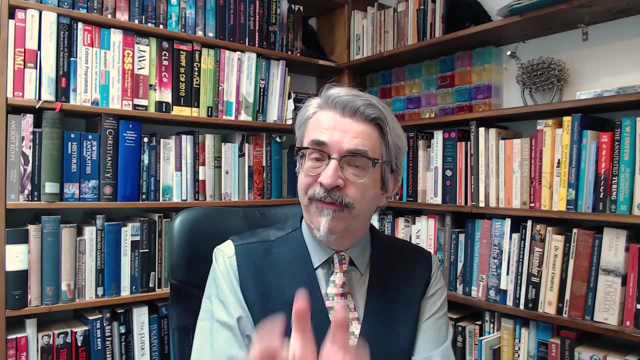 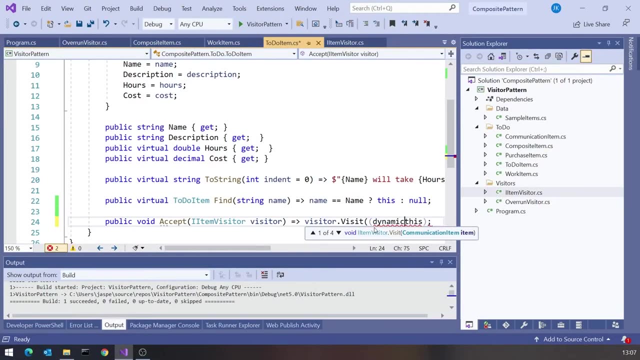 and therefore we can't make the overloading decision. But if you remember, quite a few videos back I showed you how to do what is known as dynamic overloading, where we can defer that decision from compile time to runtime And all we need to do is cast that to dynamic. 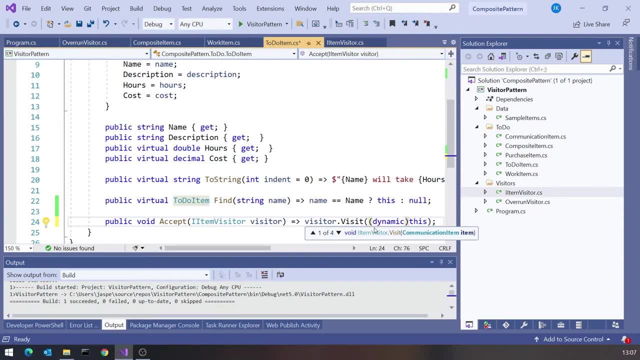 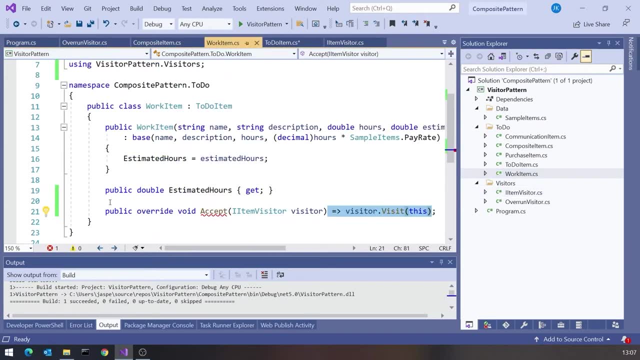 which basically means the component is spawned on top of the load tag, so to mean that the decision is done in, the compiler does not know what it is at all, And that means it has to defer to runtime. And so now we can remove all of those, just for simplification, from each of the 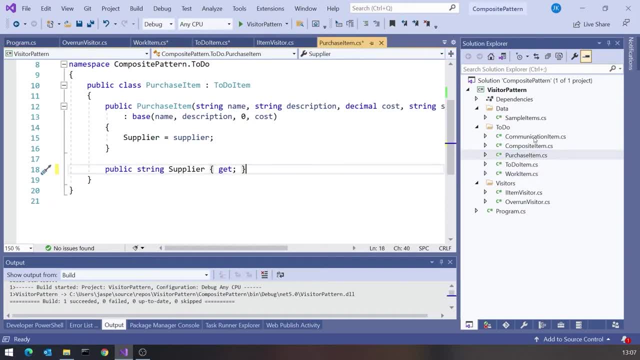 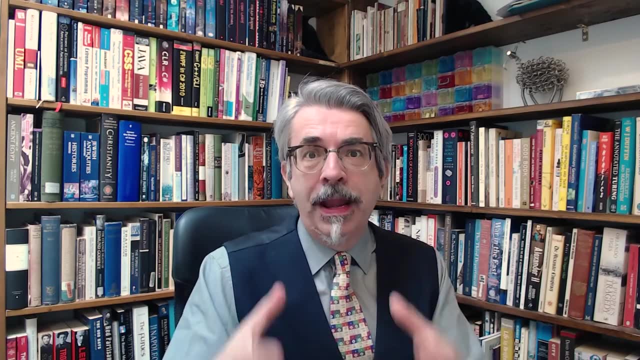 leaf nodes And it will work in exactly the same way. And it really is as simple as that. Now we can just progress on and add as many more visitors as we like. So I'll just do a couple more. Remember, on the purchase item, we had a supplier, So 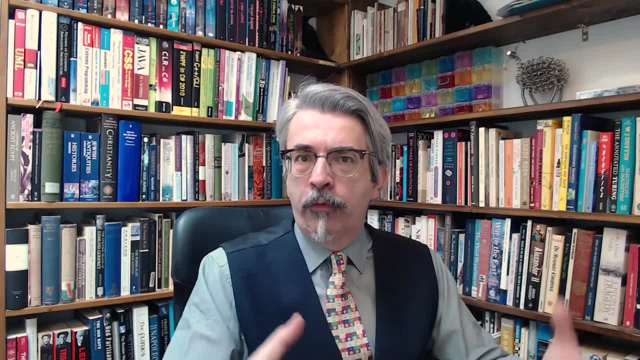 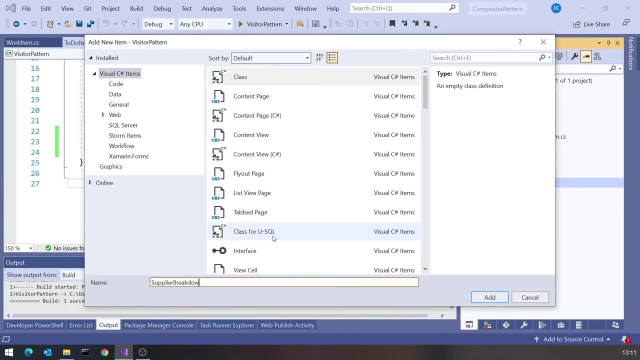 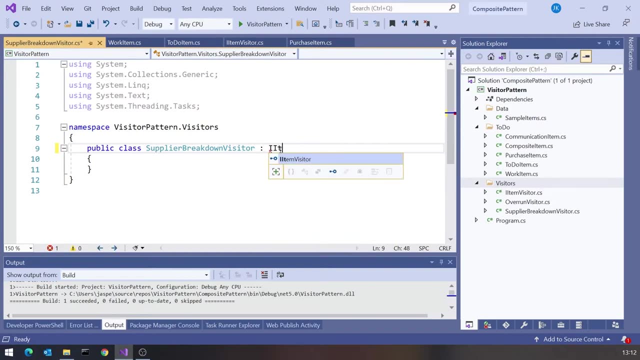 let's do a visitor that can summarize what we bought from each supplier. So we'll go in here, add a new class and we'll call this Supplier Breakdown Visitor. As ever, we need to implement the interface And in this case, what I'm. 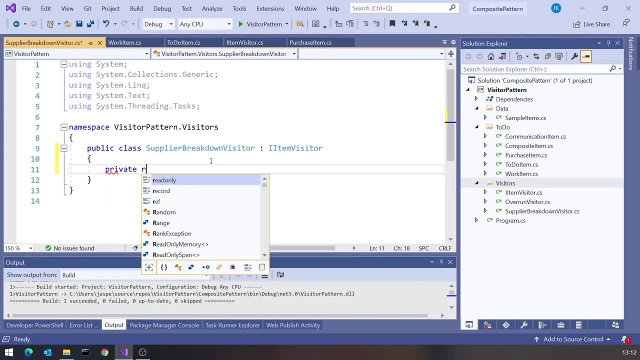 going to do is I'm going to put in a dictionary that maps the supplier name to the amount of money spent with that supplier. So we'll have a dictionary string for the supplier name, decimal for the spend. So then we're going to do our visit. So let's once. 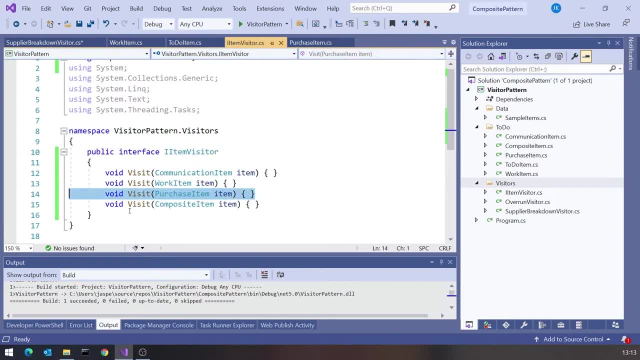 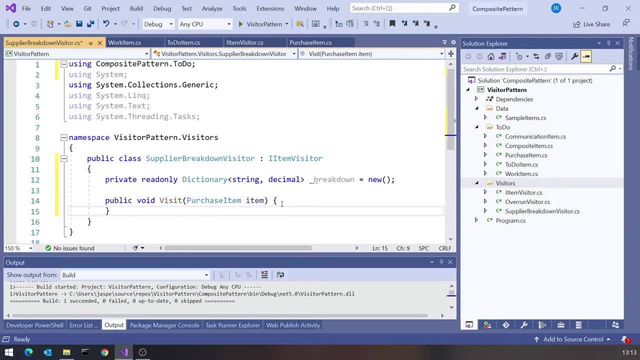 again, just steal the stub of that from our interface And then pop that in there. So what we'll do here is based on the name on that purchase item. we'll look up the supplier And then that may or may not be the first time we've had this. 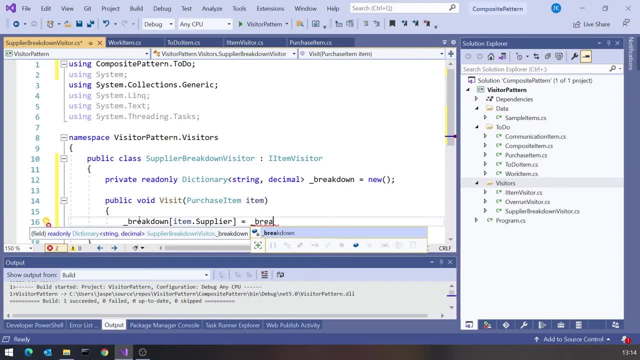 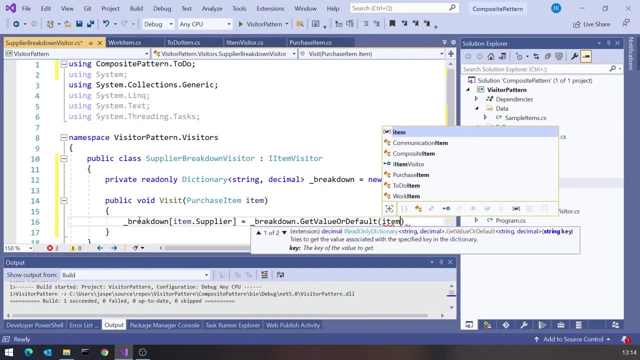 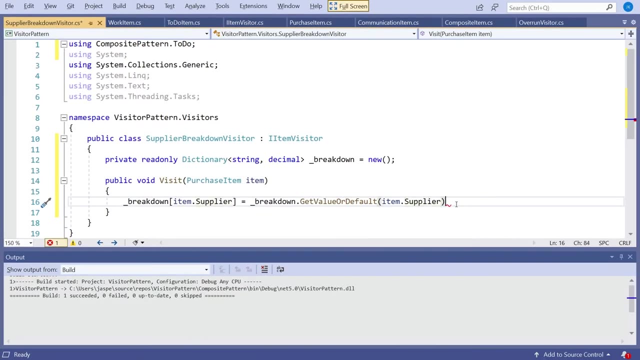 supplier. So what we can do here is, if we say breakdowngetValueOrDefault on itemsupplier, what that will do is either give a zero for the spend if it's the first time we've had this supplier, or give us the current total, And then we can merely add on to that the cost of. 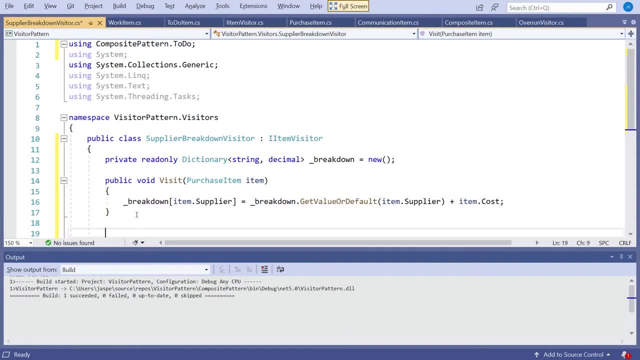 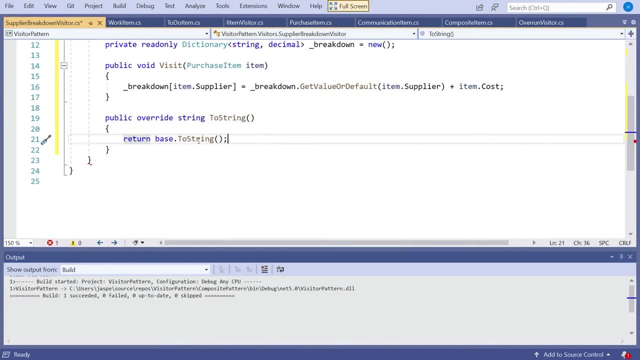 the next one. So there, we've got the addition, And then we're going to actually need just to display this. so let's just put in an override of toString And we'll use a string builder for this, And so we'll just loop through the dictionary. 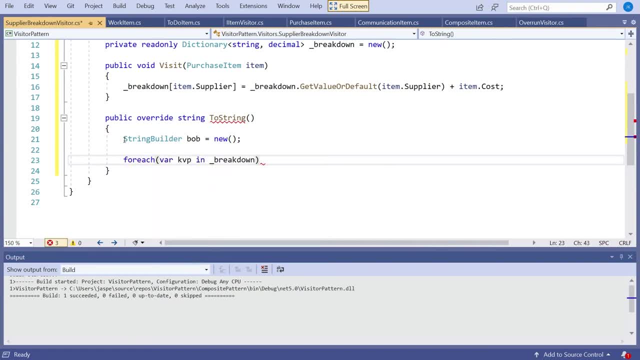 So we're getting key-value pairs out of that and we will pop on to the string builder the name of the supplier and then the cost, which is the value, And then just return the toString on that And then, once again, haven't you? 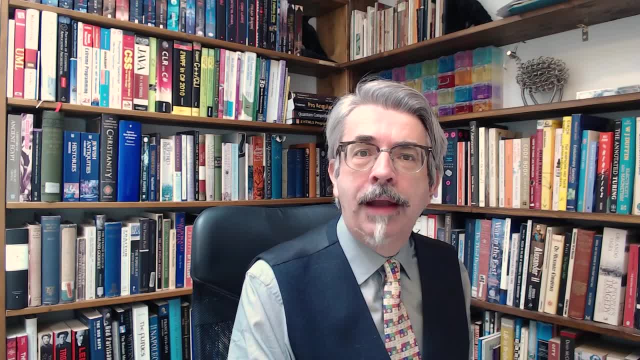 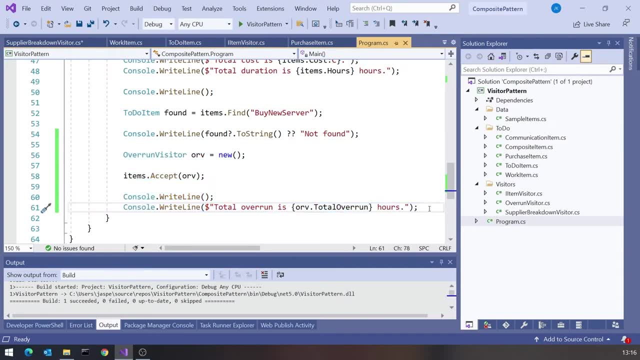 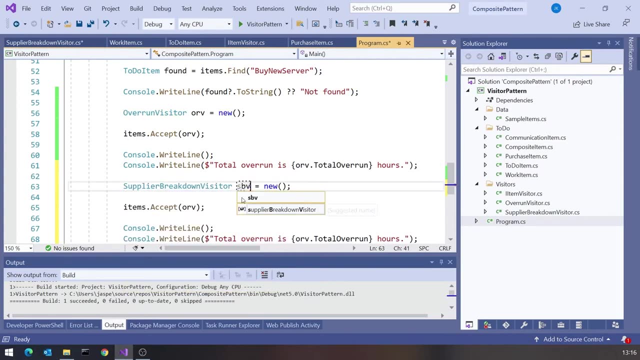 having done all that, the easy part is we just need to add that in to our program. So we'll, down here, have pretty similar to that. So in this case it's going to be a Supplier Breakdown Visitor. We'll call that SBV. We send that in to Visit and then in 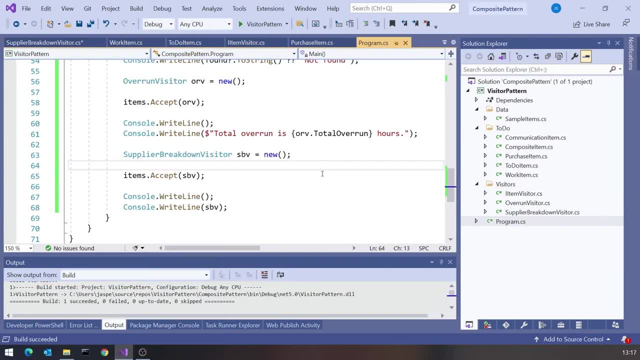 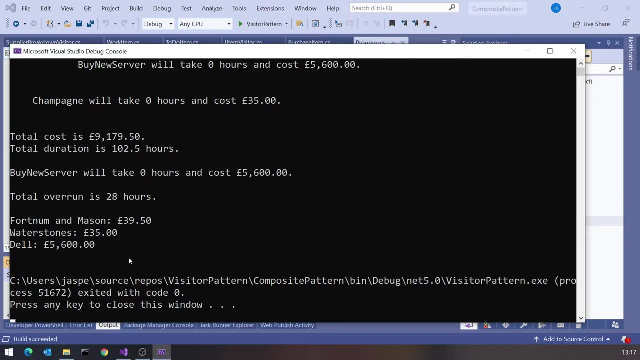 this case we can just output the toString and then run that up And we can see: we spent £39.50 at Fortnum & Mason, £35 at Waterstones, £5,600 at Dell. So again, very simple to add that. And in fact, if you want to take this to the 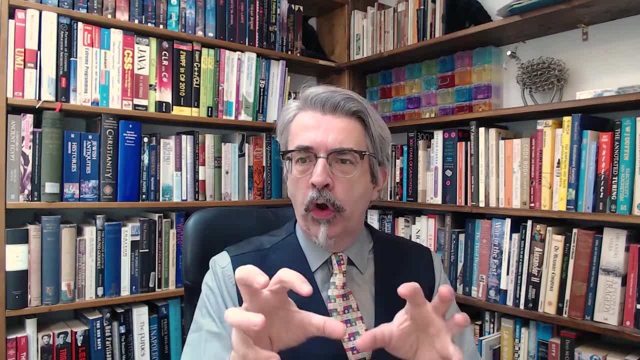 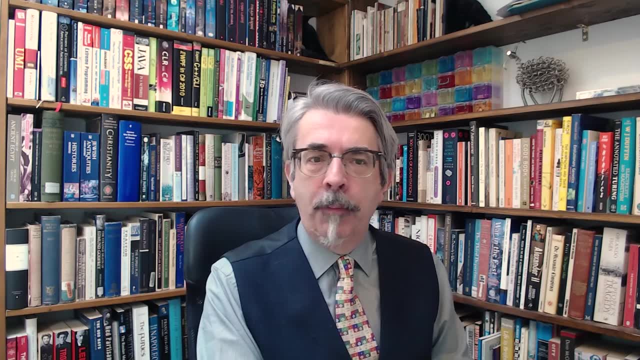 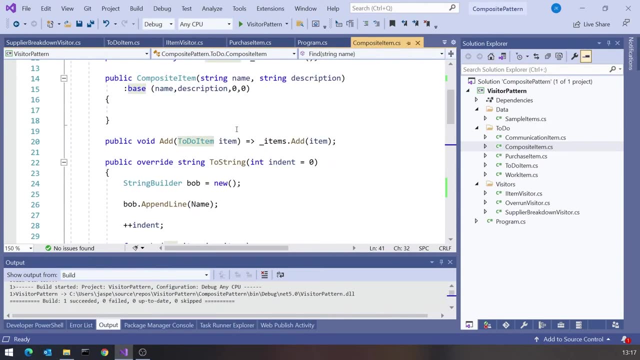 extreme, you can replace every one of the existing methods that we had with just the use of a Visitor. So if we take a look at our Composite, then we only really need to have the Accept and everything else like the Find, the toString, and all of that we could just replace with the. 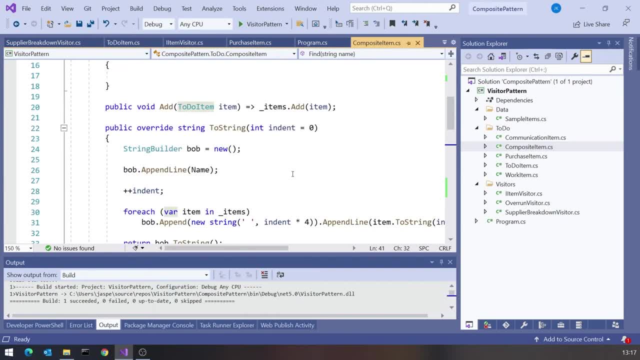 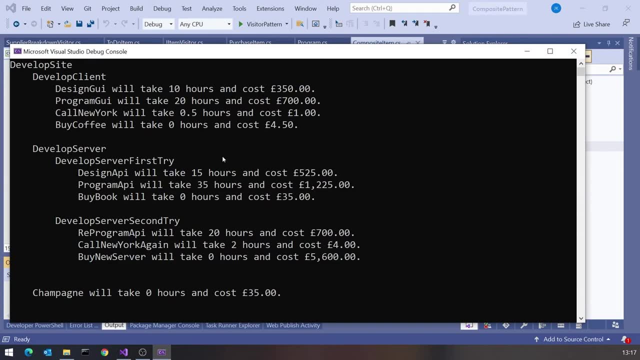 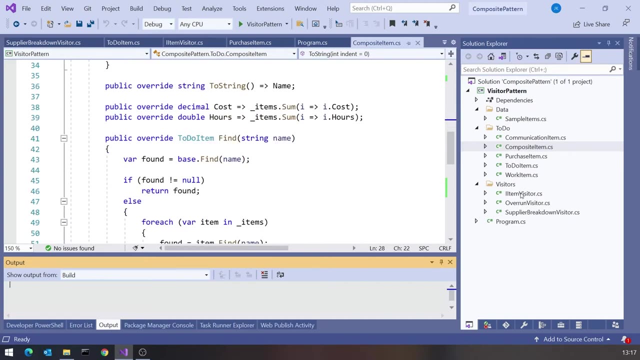 Visitor. When it comes to something like the toString, it's a bit tricky because, remember, we've got this indent on the toString that we increment each step along so that we get this nice layout that we've got here, And so we've got to be a bit tricky with that, And so the way we do that is this: We add another method. 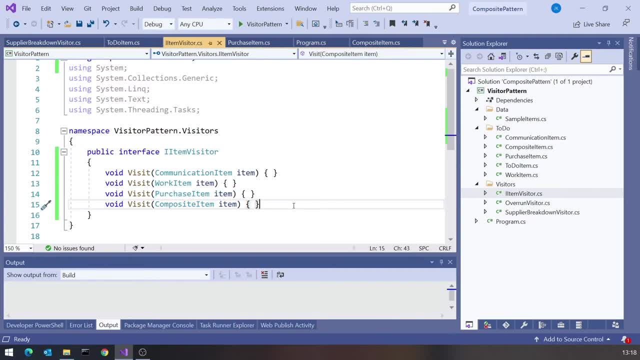 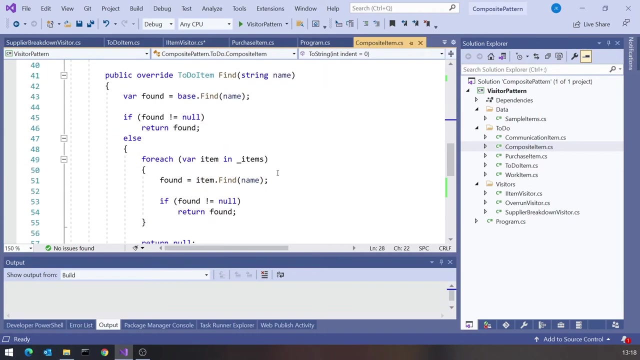 on to the Visitor interface and this returns an Item Visitor and we call this getChild and by default that does actually pretty much nothing at all, It just returns our self. But then what we have to do with that is on the Composite: rather than passing the Visitor straight down to the child, we actually create the. 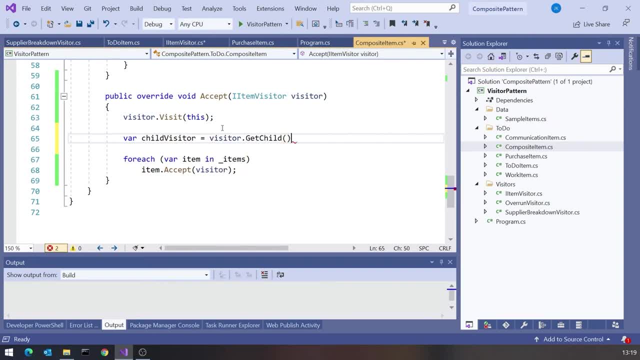 child Visitor and that's what we pass down. So we get a different Visitor with each generation down And with the Overrun and the SupplyBreakdownVisitor that doesn't matter, and so those visitors just leave the default implementation in there. But when we come to this equivalent of the ToString, that's 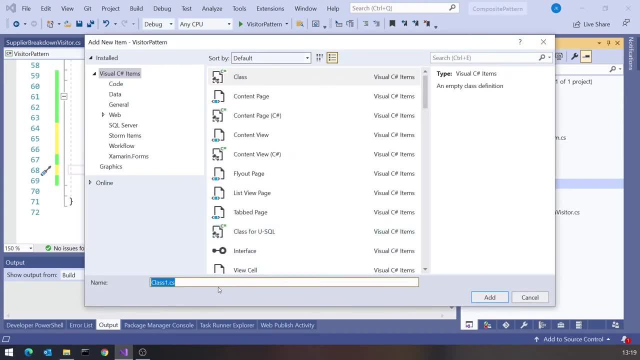 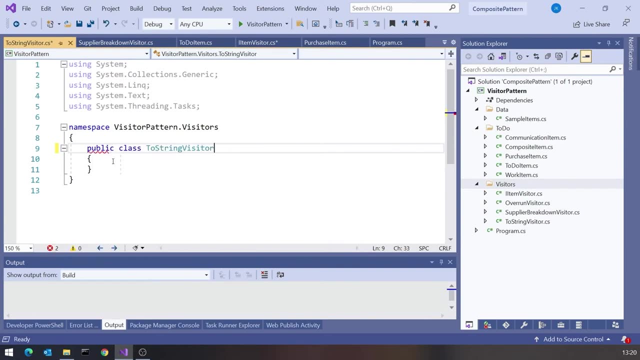 when things get a bit more complicated. So we'll put in here another class and this we're going to call our ToStringVisitor. Again, it's going to implement iItemVisitor, And then what we're going to have to have in here it's: 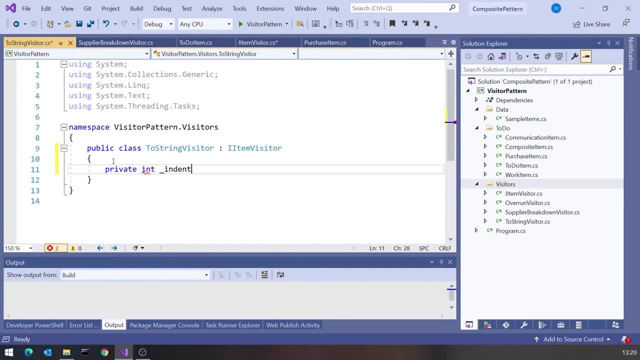 going to keep track of the indent and also it's going to have its own StringBuilder. That is what's required to put this all together. We're going to have a constructor that creates a new StringBuilder And then we're going to have an overloaded constructor, which is going to be private and which is going 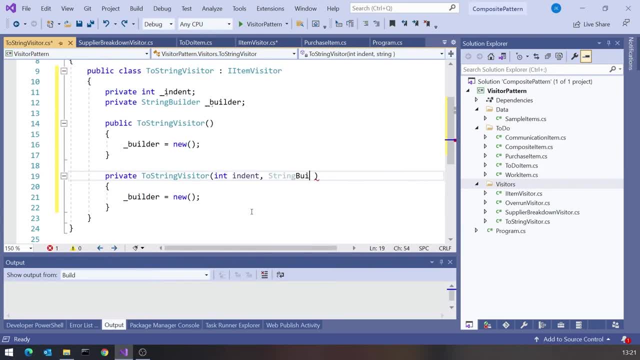 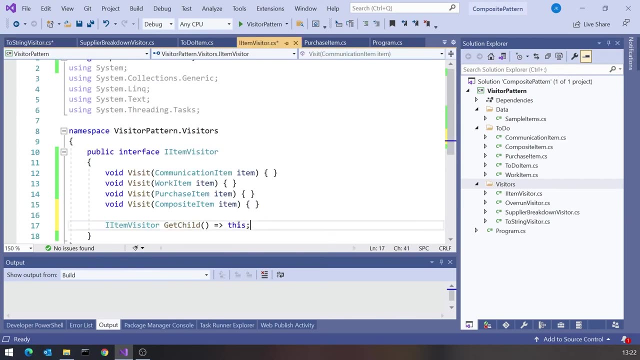 to take an indent and a StringBuilder And for each of those it's just going to set the fields to be what's passed in. And you'll notice that I've made that private because that's what we're going to use in our GetChild. So, although by default, 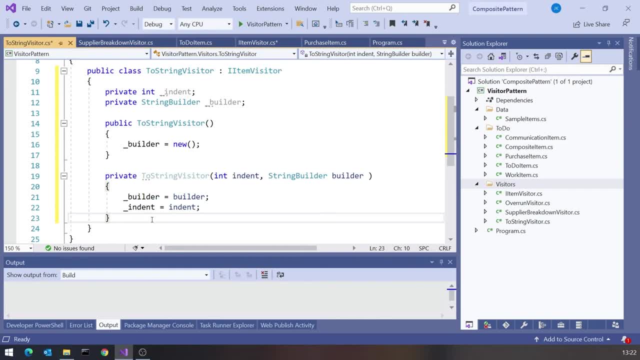 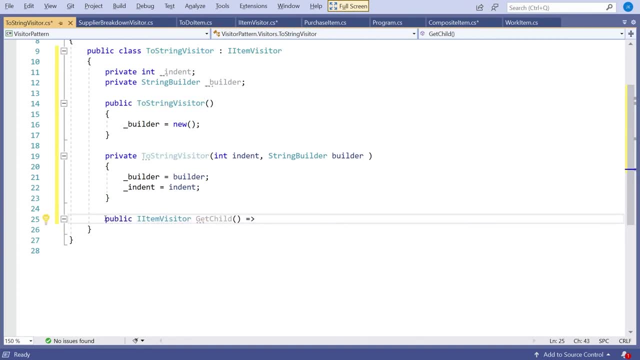 when we GetChild. it does nothing at all really. but here I'm going to have a GetChild and what the GetChild is going to do is return a new StringVisitor using that private constructor. So the indent is going to be indent plus one, and then the builder is just going to be the same builder. So 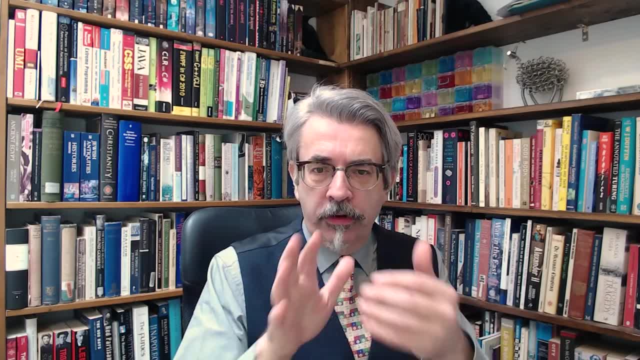 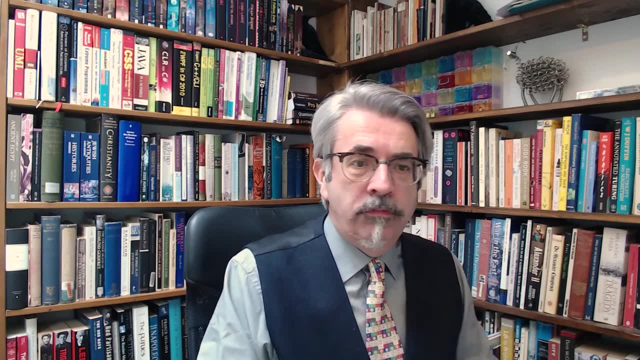 that means that every time we go down a generation, it'll call GetChild, and we will have done that to increment that indent, which is what we wanted to do before Then, apart from that, not much more we've got to do, We've got to just. 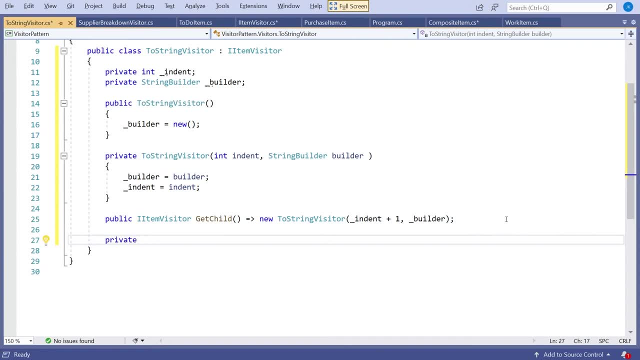 put together a little helper function. So I'm going to call this PrivateVoidantVisitor private vi-vo-id-show-string, which is going to take a to do item. So this is going to be one of the leaf nodes really, And here what we're going to do is actually steal the code. basically, they. 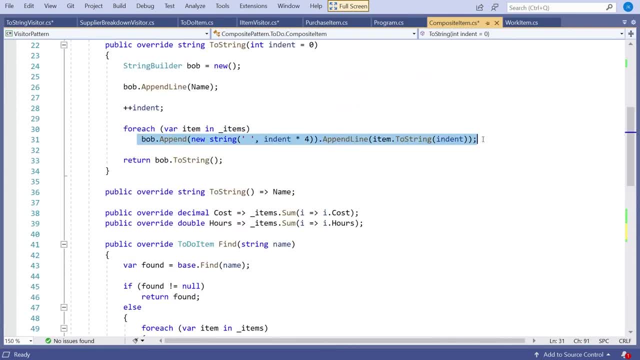 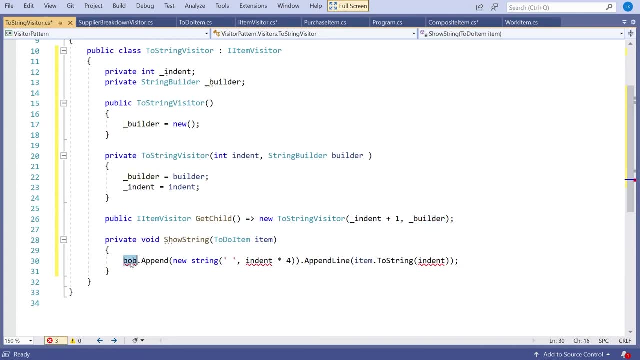 already had, which, remember, was doing that to deal with our indentation. So we'll take that, put in there, Replace the builder name with underscoreBuilder, and then we're going to multiply that, that by underscore indent, And then we're just going to have the toString called. 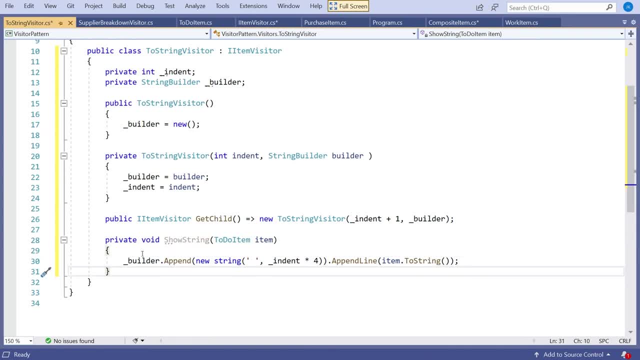 directly on there. So that's showString. And then we're going to have to now implement all of the methods in the visitor interface. So we'll take all of those and just pop them down there, Make them public, And then all they're going to do. 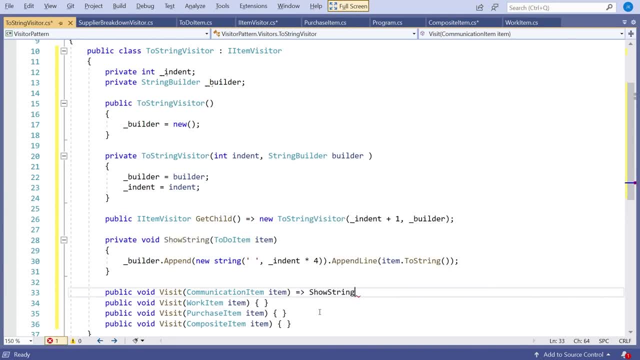 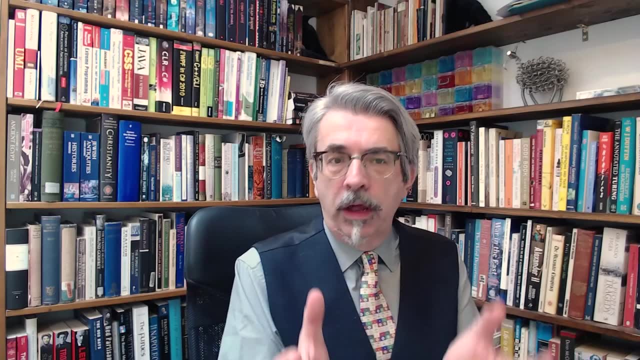 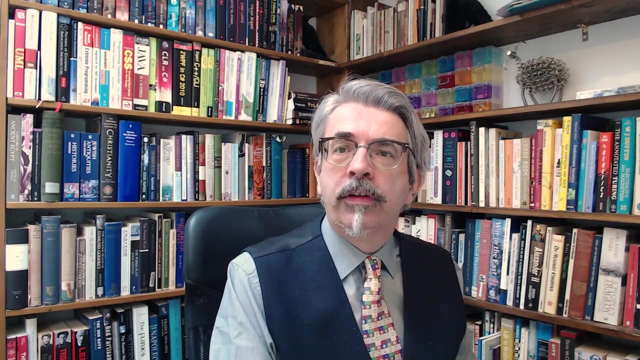 is call that showString on the item itself, And that really should be. it So slightly more complicated one there, partly because it's the first one of these that's going to have to generate a child. But now, if we do that, let's just 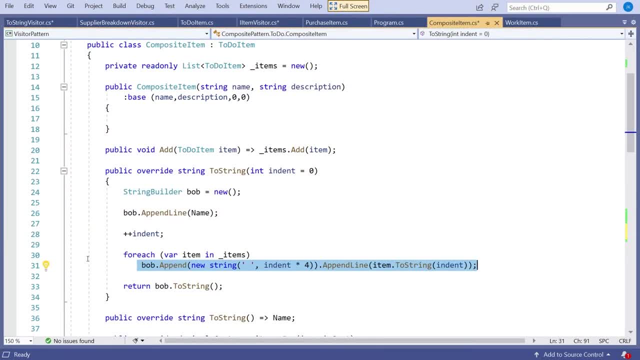 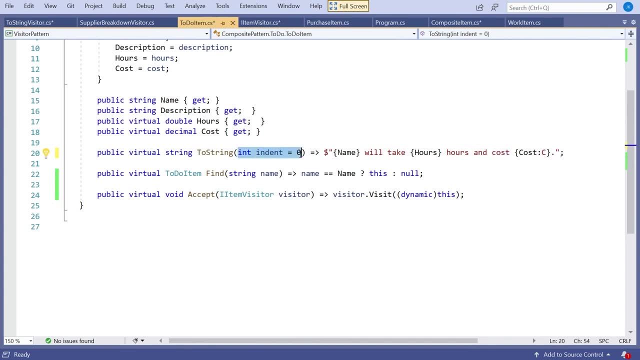 now get rid of the toString that we already have on the composite and also change that on our base so it no longer takes the indent on there. So this is is now actually back to overriding the original toString, And then in our program we'll just do another one of these. So this is going to be our. 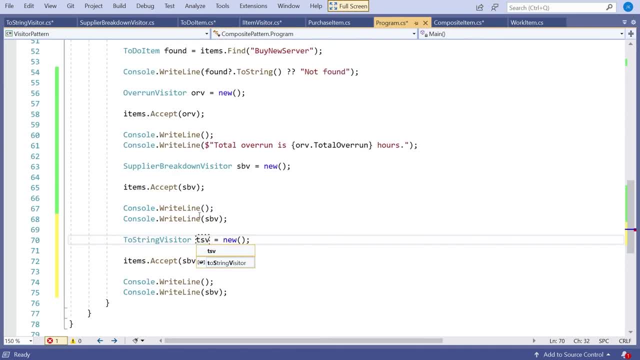 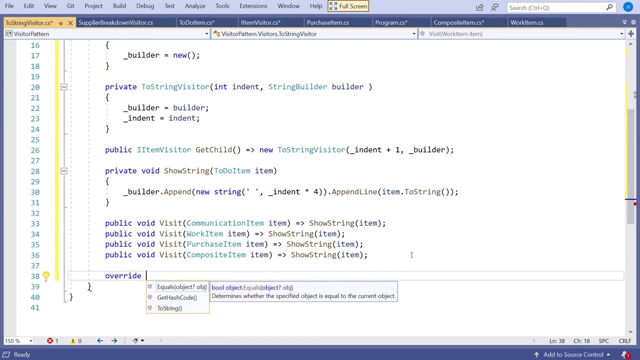 toStringVisitortsv. Just remember, actually we need one more thing on the toStringVisitor, which is it needs its own toString so we can actually see what's in the builder. So if on here we just do an override of toString and then all that needs to do, 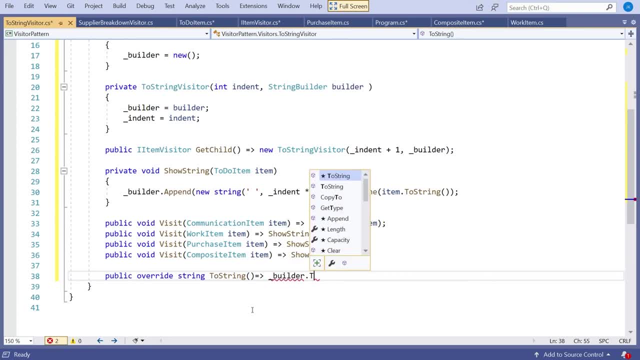 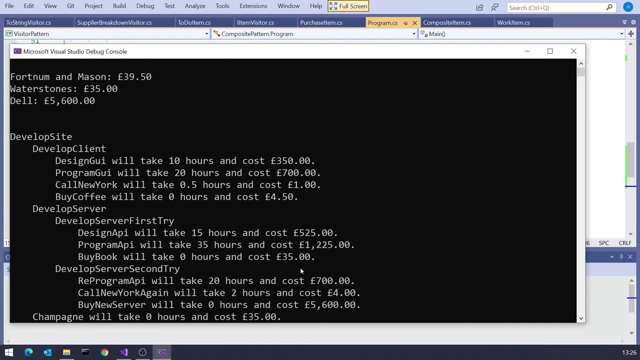 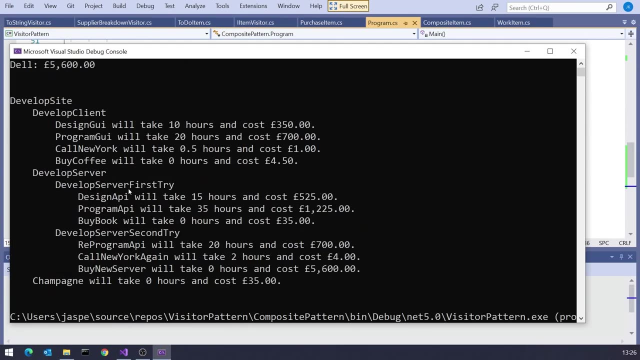 is return underscore builder, And so that's what will get called when we do the write line on tsv And when we run that we can now see right at the bottom. so after we displayed that, this is where we're using our toStringVisitor and getting exactly the same result. So 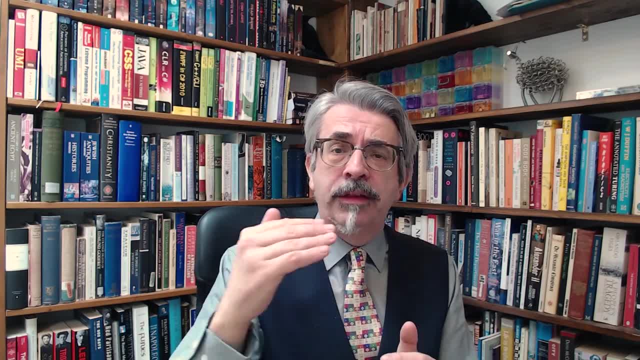 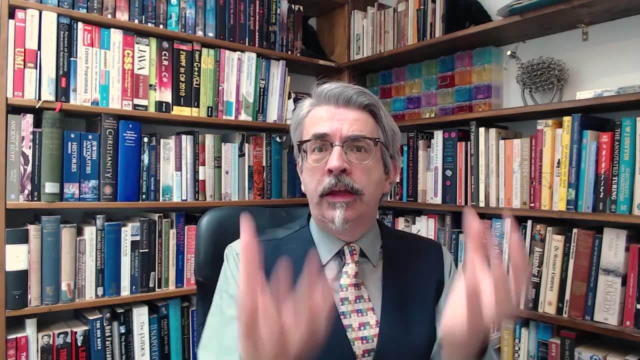 that's it. There's the visitor structure. We just have this visitor interface that has a visit method for each one of the leaf nodes that you can default to do nothing at all if you want to. And then on the composite structure, we have the accept method on the toDoBaseClass that takes a.